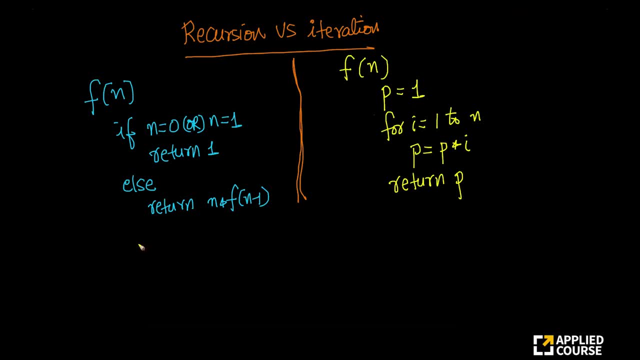 So now let us understand the fundamental difference between recursion and iteration. So we have seen the recursive function for factorial in the previous video. So and what is the time complexity and space complexity here? My time complexity is: t of n equals to constant plus t of n minus 1, which is equal to big O of n. What is the space complexity? 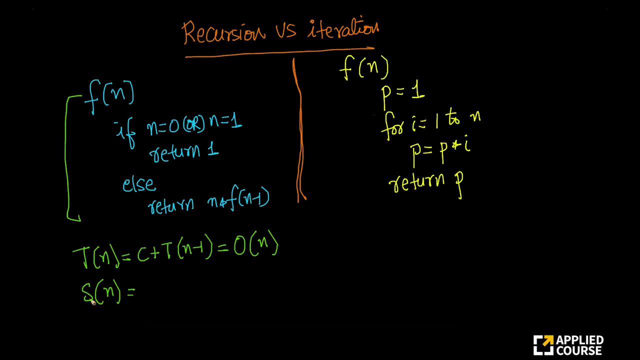 What is the space complexity? So let us write t as time complexity, s as space complexity. Space complexity was also order of n, primarily because of call stack. That is important, primarily because of call stack. here. Now, the same thing, same thing if I implement: 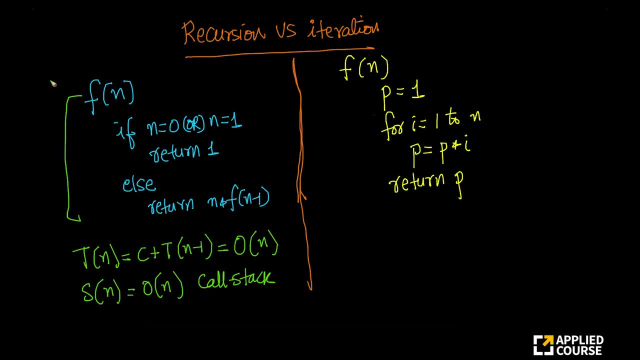 look at this same thing if I implement with iteration. So this is recursion, So this is recursion And this is iteration, This is iteration. Now, one thing that you will notice is when you are writing an iterative algorithm in iteration there is no, so here, 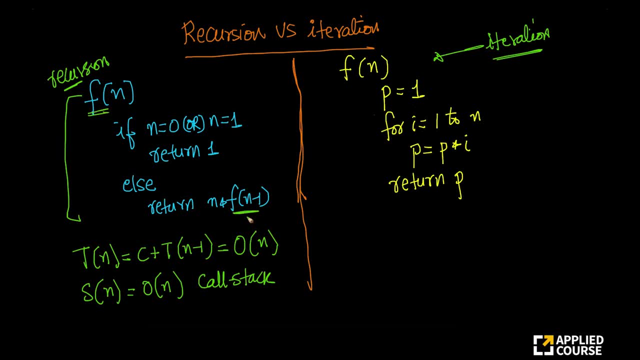 why is it recursive? Because I am calling this function. I am calling the same function with different input values here. Here I am not calling the same function, fn. This is also to compute factorial. What am I saying? I am creating a variable called p which stores the product, For i equals to 1 to n. p is. 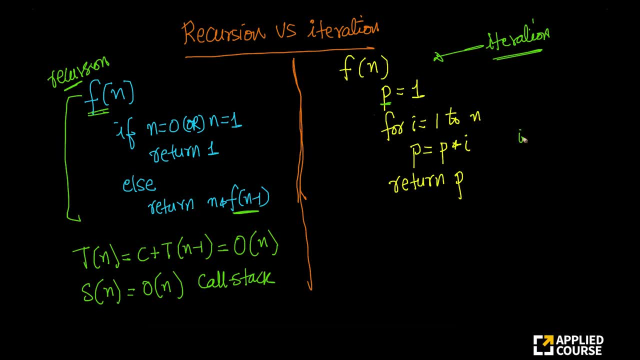 p into i. So what is happening here? My i is my p initially, is 1 into 1.. As i gets incremented it will be into 2, into 3, up to n. So this is the iterative definition of what a factorial is. Then finally, I am saying return p. 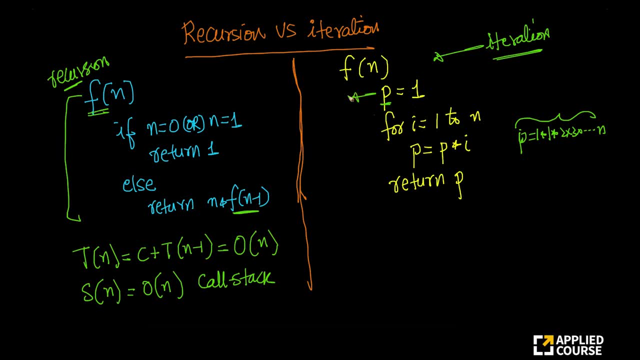 What is the space complexity? What is the time complexity for this? This is constant. This is constant, but this loop runs n times. So this whole thing will be c into n, And this is constant. So time complexity of this. let us call it t dash. n is also order of n. 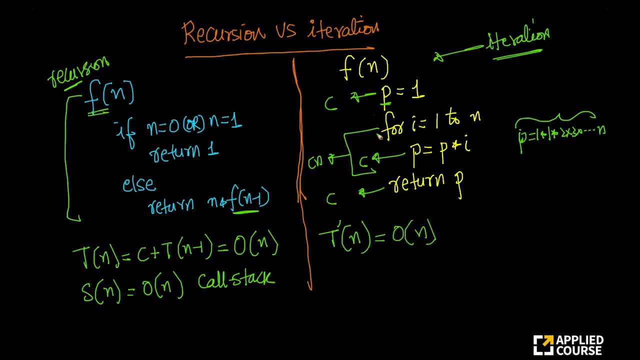 Okay, nothing changes, Because this step is run once, this step is run n times because of this for loop, because of this for loop, Right. That is why this is c n, this is c, So the total time complexity is very straightforward. nothing different, Okay. 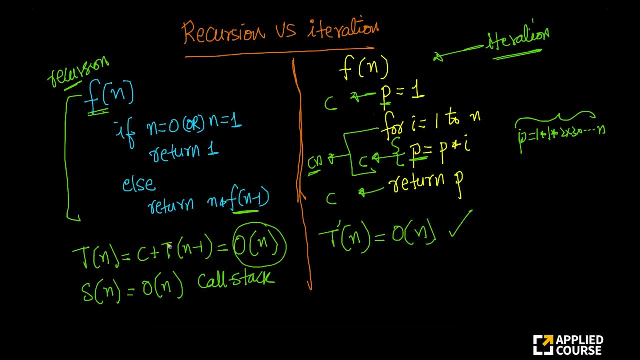 one thing you have to notice is this: space time complexity using recursion and the time complexity using iteration are the same, Right. But now let us come to the space complexity. Let us write it as s dash n Right. So what is the space complexity here? Look at this. I 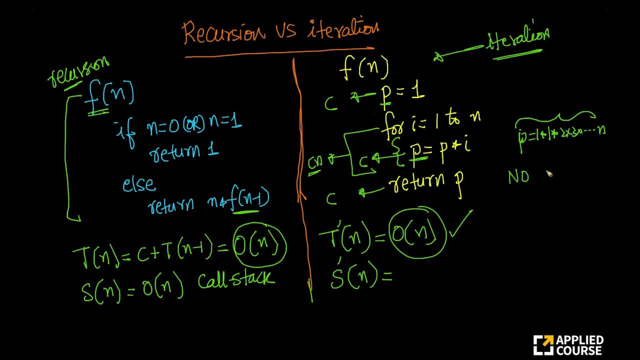 do not have any call stack here. There is no call stack issue. I do not have to bother about call stack because I am not calling the function within a function type of setup. I am creating a new variable called p. I am creating a new variable called. 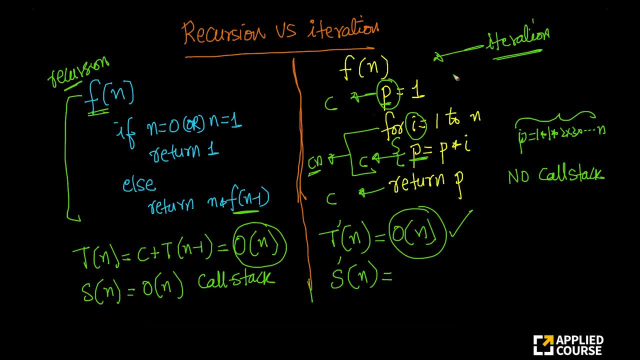 i, Nothing else. There are only two variables that I created, Right. So what is the space complexity here? It is order of 1.. Right, This is a very fundamental difference between recursion and iteration. In recursion, because you have the call stack your space complexity. 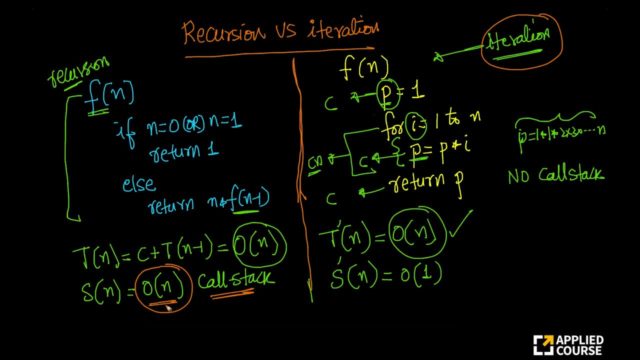 especially for this function is order of n Right. So this is an order function. You see, you are obtaining the same result here. The time complexity is exactly the same, but the space complexity here is significantly less Right. This is a very, very fundamental difference. So a lot of times when you have 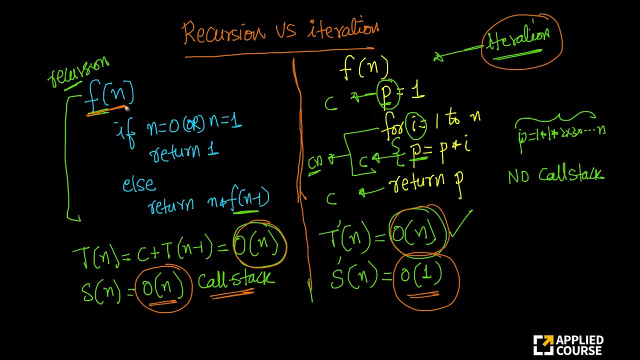 a recursive function. not a lot of times. sometimes, actually, I should say Sometimes- if you have a recursive function, you might want to convert it to iteration. if it is possible, Okay, You might want to convert the recursive function into an iteration if recursion is. 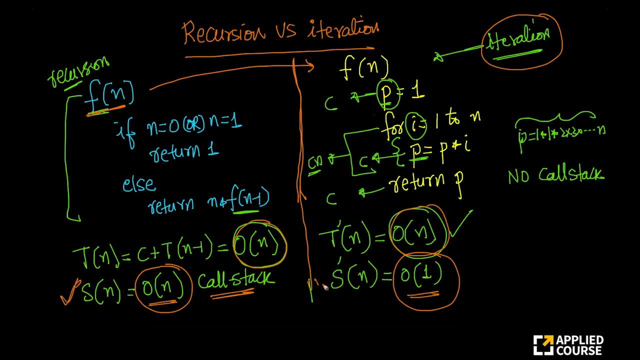 function to have better space complexity because there is no call stack issue. okay, we will discuss an interesting idea called tail recursion little later. okay, we will. we will understand a call concept called tail recursion which enables us to reduce, this time from the space complexity using a very nice hack. 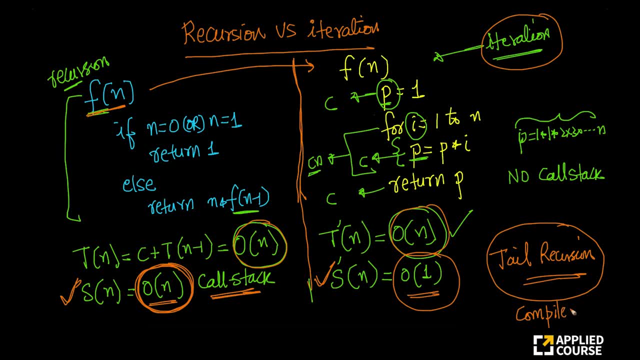 that most compilers, that most compilers actually enable us to do, most modern compilers, I should say so. there is a way to modify recursion itself to reduce this order of n call stack. okay, we'll learn that in one of the next videos, but for now the important thing is if it is easy and if it is possible and if it's. 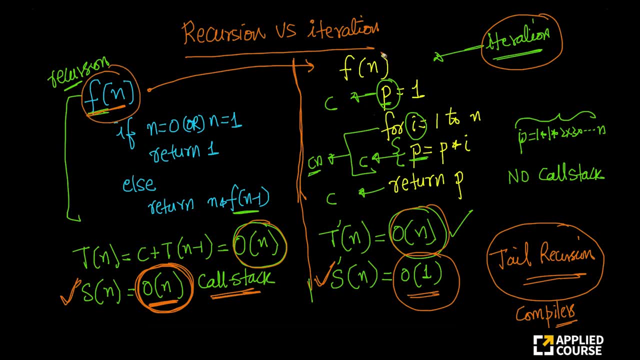 simple right to convert a recursive function to an iterative function. you should always prefer an iterative function because there is no call stack issue that you have to bother about right this? this is an important lesson in general. of course there are some programs. this is an important lesson in general. of course there are some programs. 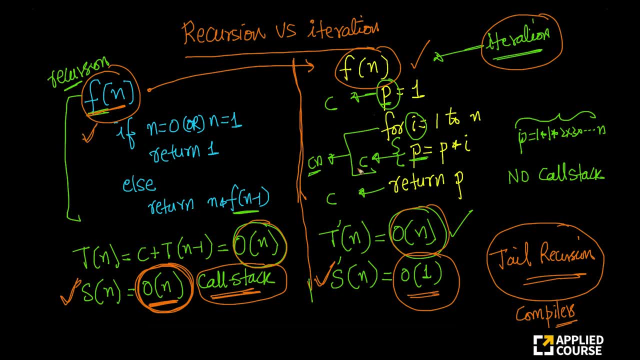 which are much harder to convert from recursion to iteration, as we'll see later in the course. right, of course, every recursive function can be converted to iterative function, but the process may be harder. you might have to write many, many more lines of code which are more prone to errors. 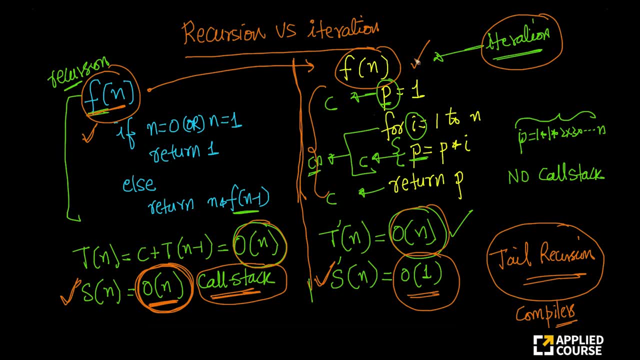 when you write iterative code for recursion, right. so sometimes people are like, okay, i don't care, even if there is a call stack issue, i might want to write recursion because the code is simpler, the code will work better and there are going to be lesser number of bugs in recursion. 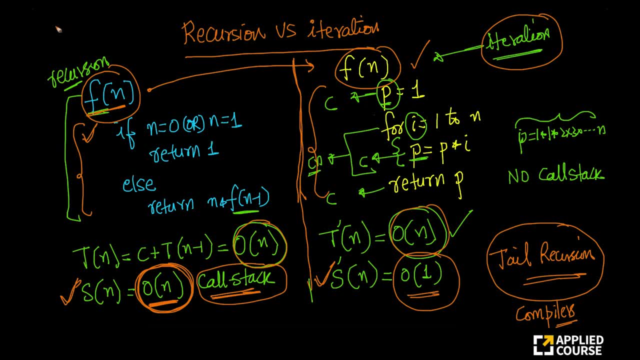 and this is easier to understand in some instances. okay, we'll learn of ideas little later in this. in this course, we'll learn of ideas like dynamic programming. don't worry if you don't know what dynamic programming is. so we learn of a way of designing new algorithms called dynamic. 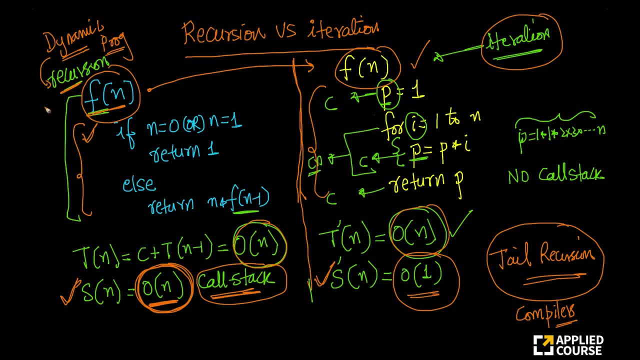 programming which uses recursion extensively. in those instances it's much easier to write your code as a recursive function, even though there is a call stack issue, than to write it as iterative. because writing it as iterative, i mean there's going to be very, very prone to errors and it's much more easy to read and understand recursive code sometimes. 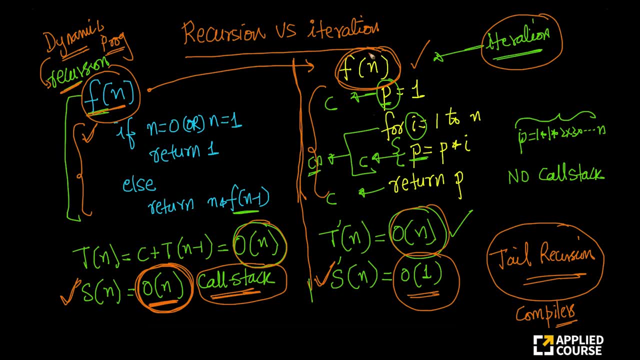 right. so there are pros and cons of both recursion and iteration. recursion is simpler to understand in some situations, but of course there's a call stack thing that you have to be careful about. iteration might require more code in some instances and you have to be careful to avoid. 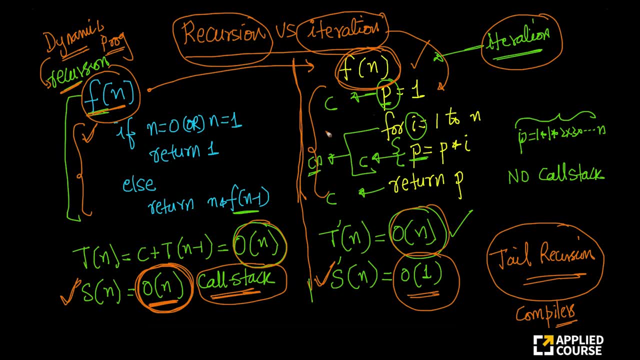 any boundary case mistakes and things like that. right, but otherwise. otherwise, this is good. oh, here, actually, i forgot to write a boundary case here. see, as i told you, the boundary case here is: if n equals to 0 or n equals to 1, return 1. right, there is this boundary case that i forgot to write. 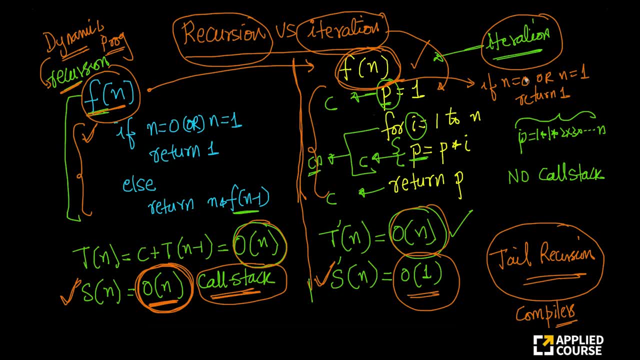 when i was telling you the boundary case, right right before p, you can say: if n equals to 0, actually this code will work. if n equals to 1 also, then the for loop will be 1 to 1. everything will work. but if n equals to 0, this for loop won't work. okay, it will not be able to return.